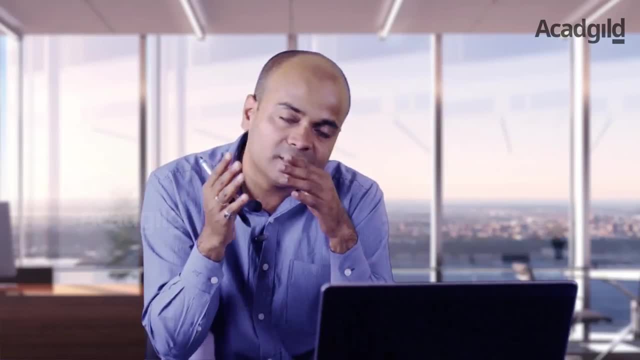 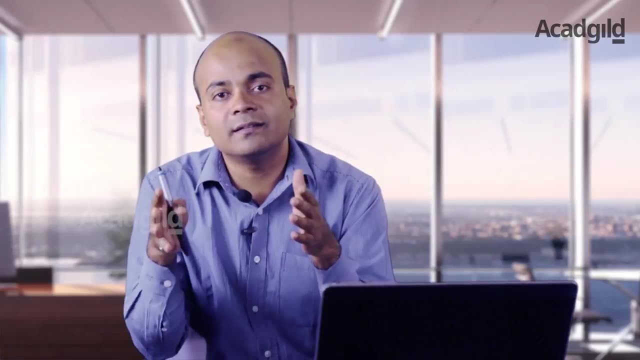 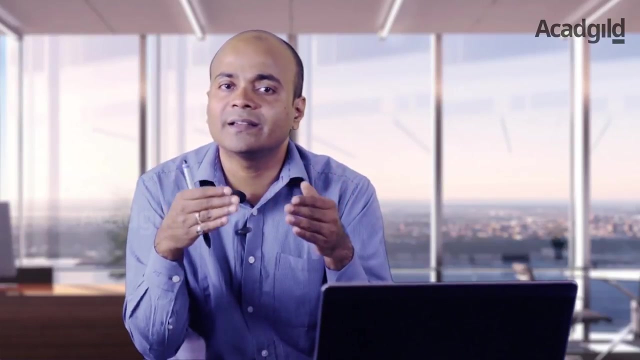 clerk selling company and you want to send a campaign to your customers, To a certain set of customers you send a campaign. To others you don't, And you want to know whether the customers are going to buy based on campaign or not, whether the campaigns were effective. 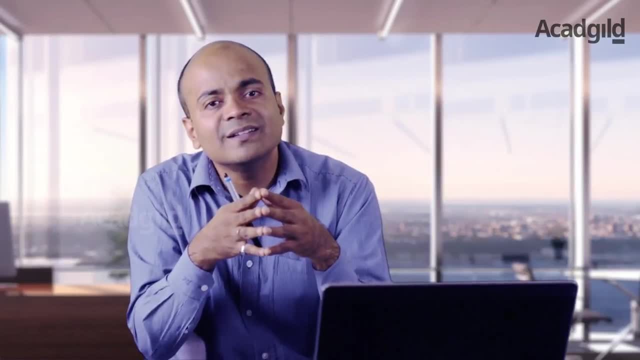 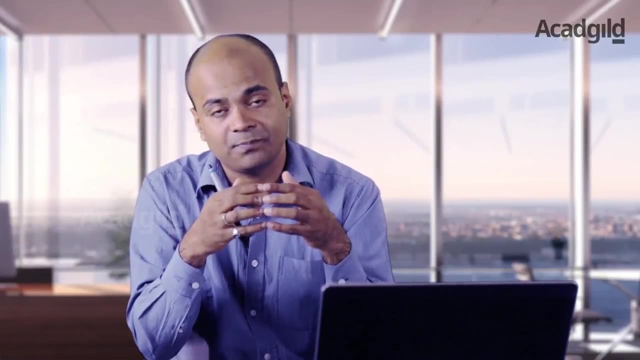 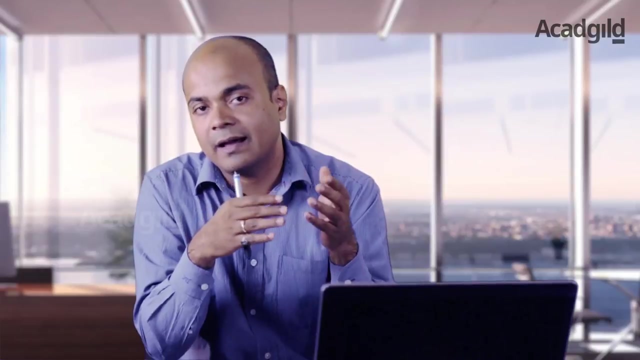 or not? Then how do you design that experiment? How do you design whom to send, whom not to send, How do you figure out how many of them to send? And once it has happened, and suppose the customers who got the advertisement clicked on it and purchased a little more as compared? 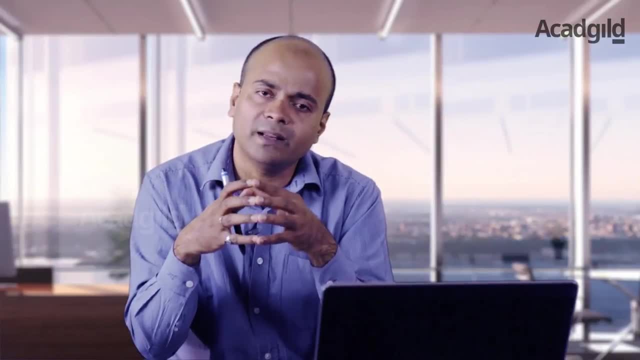 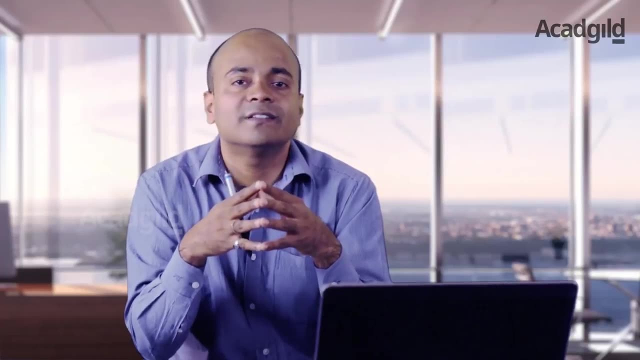 to the customers who did not get the advertisement. Now how do you establish that, even if the advertisements were not sent to the customer, the customer would have still bought. those particular set of customers would have still bought more. To answer all these questions, 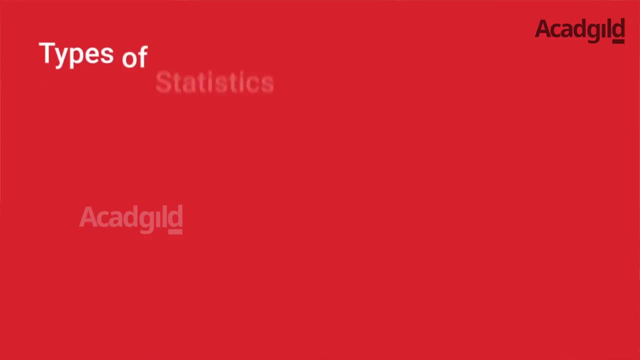 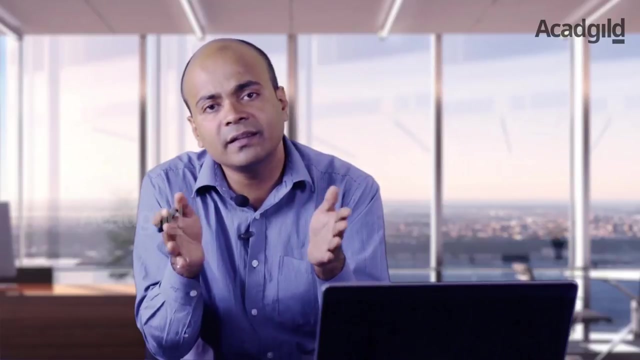 we do statistics. There are two kinds of statistics. One is descriptive statistics and the other is inferential statistics. Descriptive statistics is a method of organizing, summarizing and presenting data in the informative way. You have all the data you know, like how your business 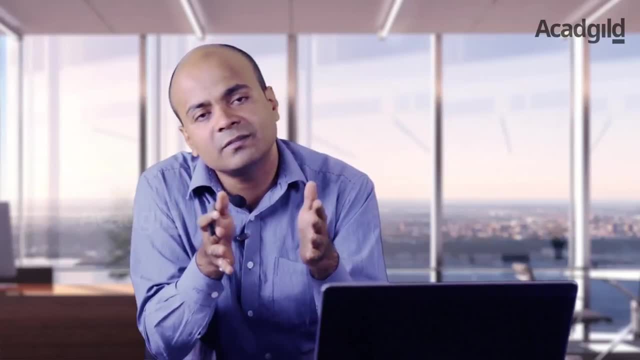 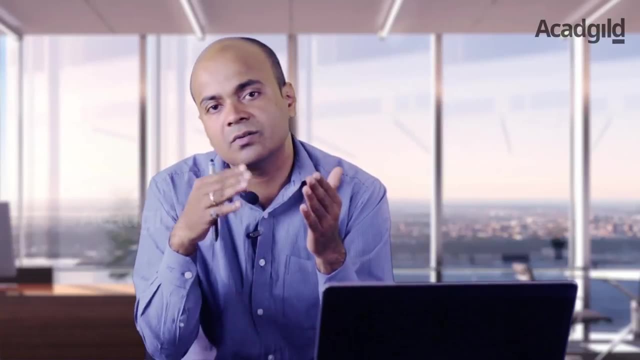 has been going on, how much inventory you keep, how many customers come to your store, in which month has it been more? on what day of the week it occurs more? which product are usually sold more, at what point of time? So there are two kinds of statistics. One is descriptive statistics and the other is 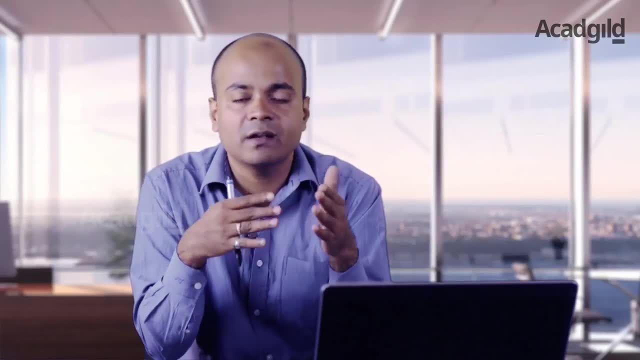 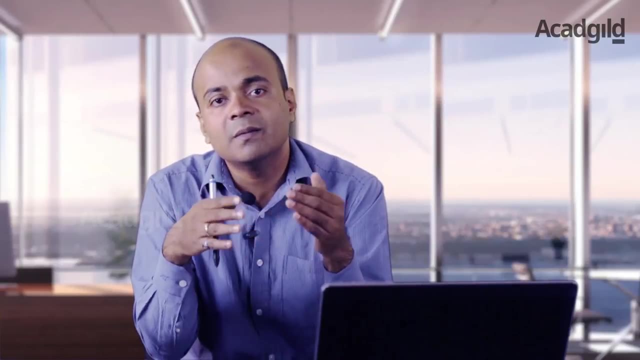 inferential statistics On what hour is your product sale more? what kind of customers come? is it like female customers come more at this point of time or male customers come at more this point of time? people with children come more. cigarette buyers come more beer. 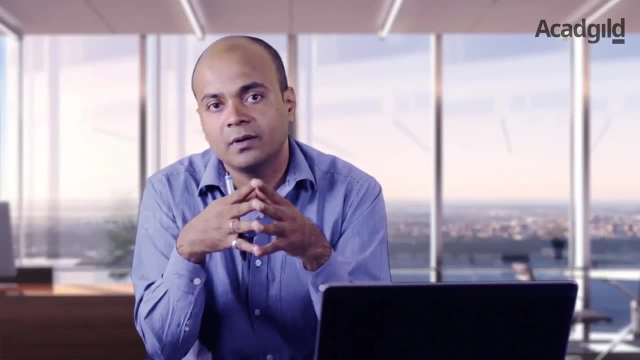 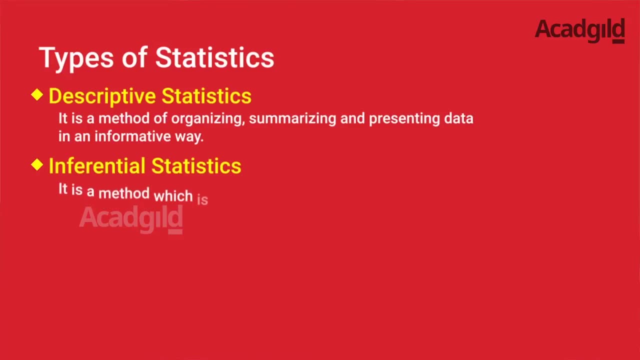 buyers come more, or grocery items buyers come more? All these questions, based on data, are answered by descriptive statistics As opposed to inferential statistics, which is a different kind of statistics altogether. you can see that the population is more than one person. Recently, we had an election. 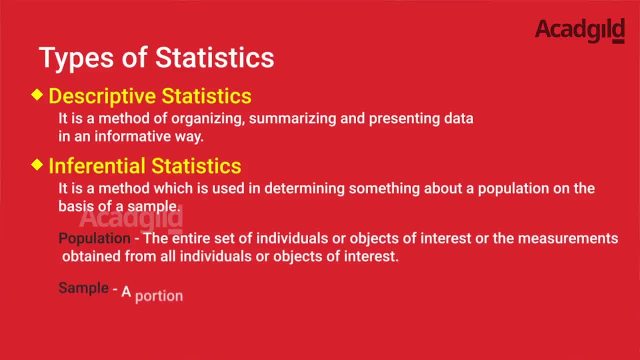 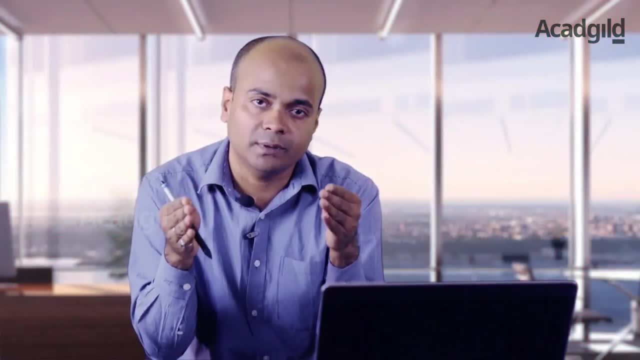 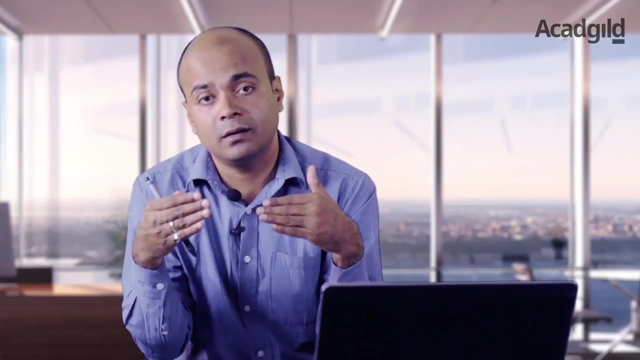 in a state. Now you are not going to ask every person whether they voted for one party or the other, But you want to figure out. So you select a sample, You decide the sample size And based on that sample size you try to infer which party is going to get more. 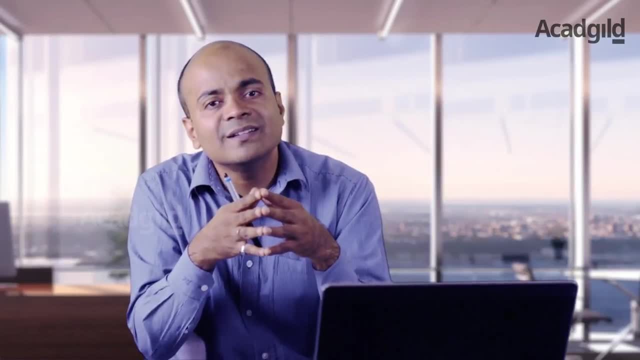 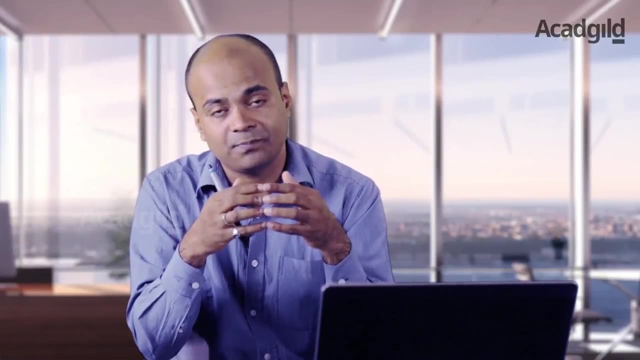 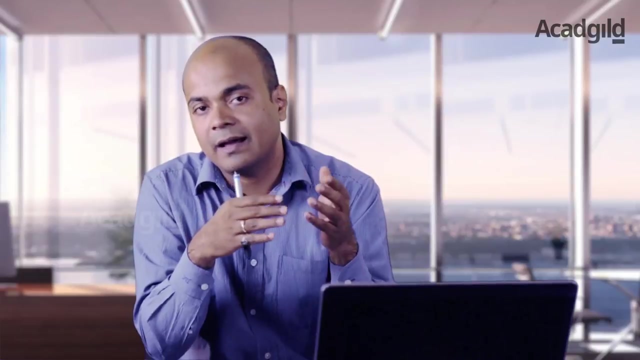 or not? Then how do you design that experiment? How do you design whom to send, whom not to send, How do you figure out how many of them to send? And once it has happened, and suppose the customers who got the advertisement clicked on it and purchased a little more as compared? 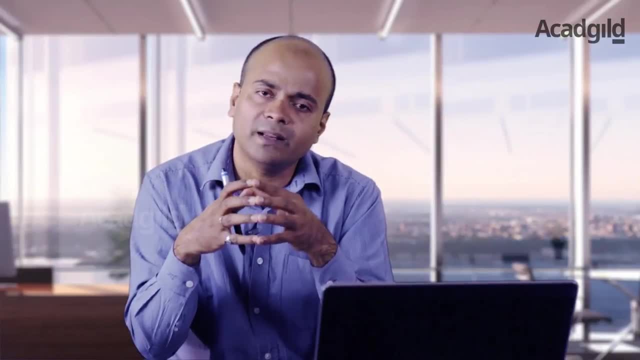 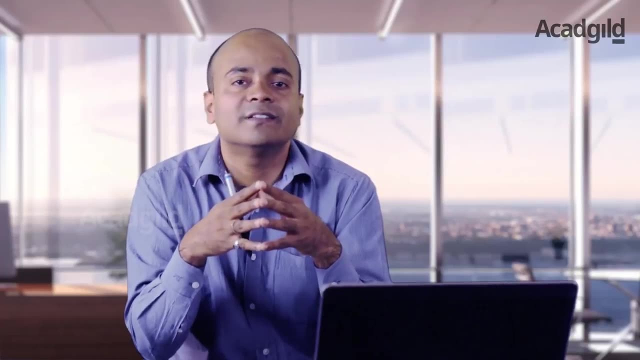 to the customers who did not get the advertisement. Now how do you establish that, even if the advertisements were not sent to the customer, the customer would have still bought. those particular set of customers would have still bought more. To answer all these questions, 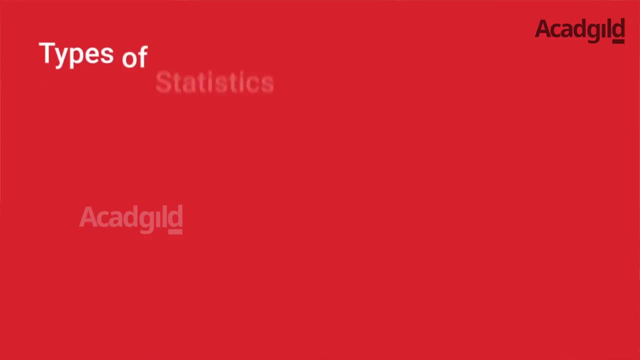 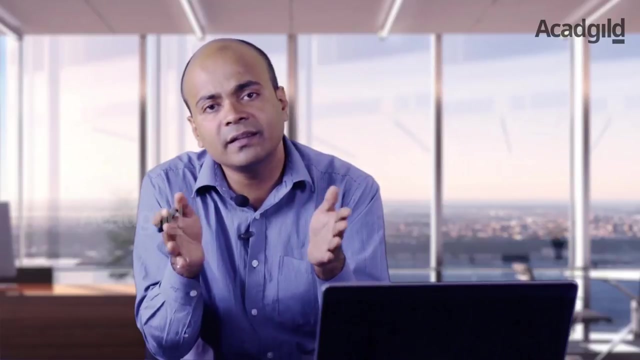 we do statistics. There are two kinds of statistics. One is descriptive statistics and the other is inferential statistics. Descriptive statistics is a method of organizing, summarizing and presenting data in the informative way. You have all the data you know, like how your business 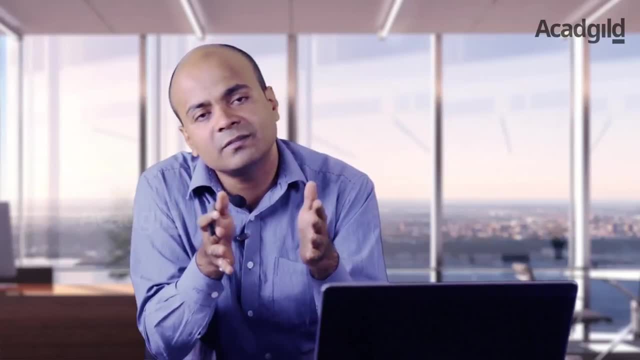 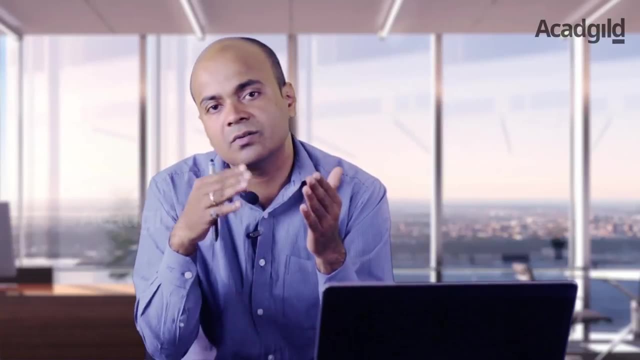 has been going on, how much inventory you keep, how many customers come to your store, in which month has it been more? on what day of the week it occurs more? which product are usually sold more, at what point of time? So there are two kinds of statistics. One is descriptive statistics and the other is 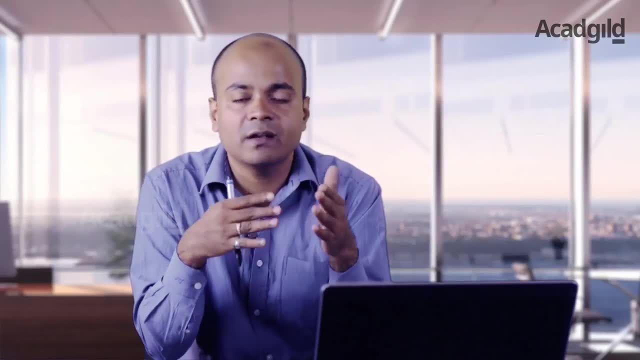 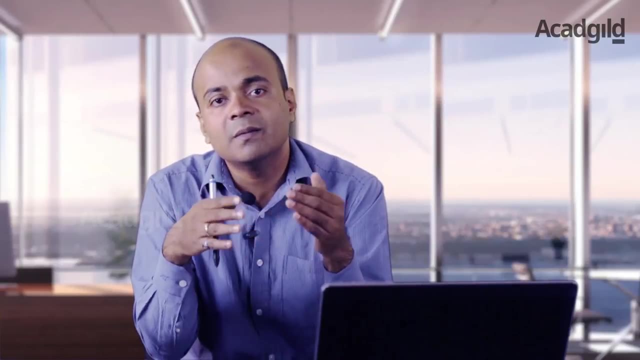 inferential statistics On what hour is your product sale more? what kind of customers come? is it like female customers come more at this point of time or male customers come at more this point of time? people with children come more. cigarette buyers come more beer. 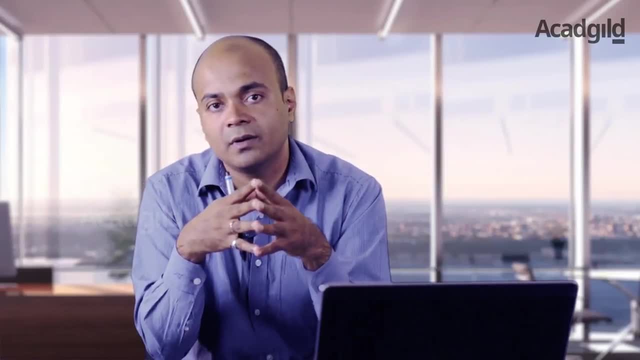 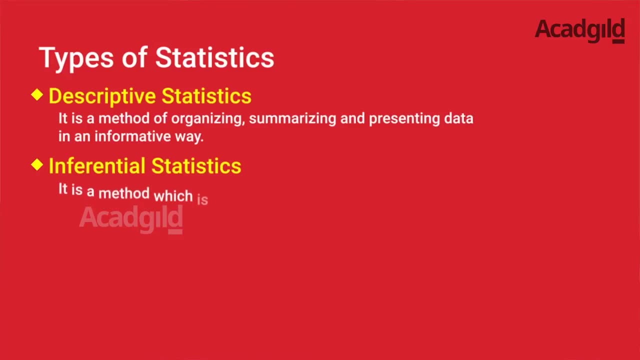 buyers come more, or grocery items buyers come more. All these questions, based on data, are answered by descriptive statistics As opposed to inferential statistics, which is a different kind of statistics altogether. it is a different kind of statistics. Recently, we had an election in a state. Now you are not going to ask every person whether 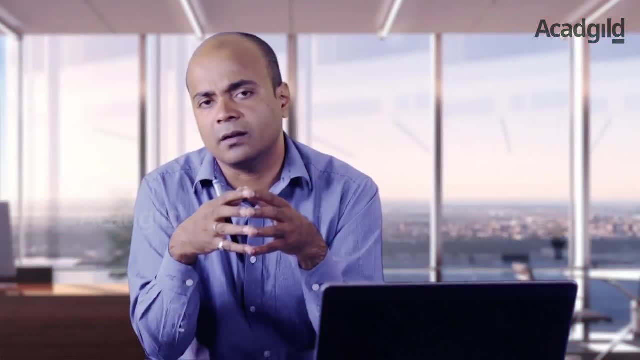 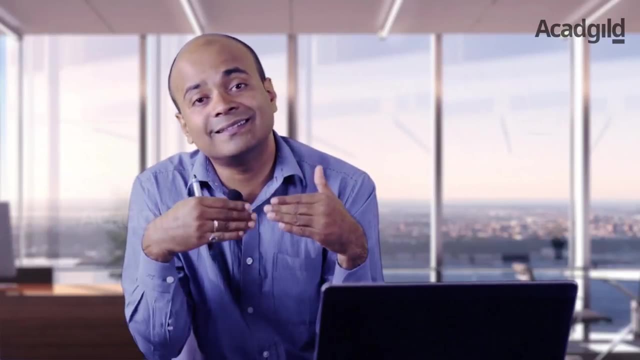 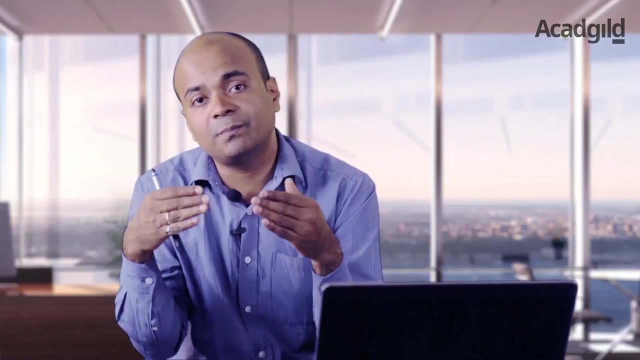 they voted for one party or the other. But you want to figure out. So you select a sample, You decide the sample size And based on that sample size, you try to infer which party is going to get more votes. You try to infer whether a person is lying or telling the truth. 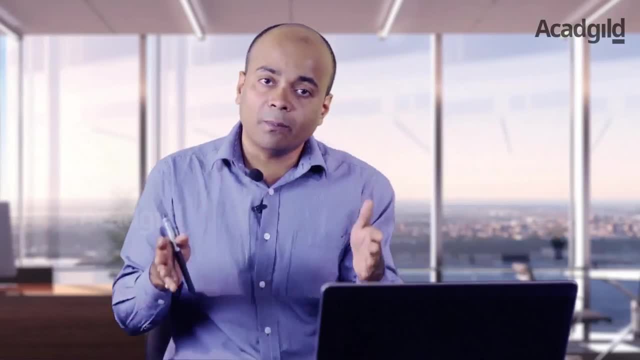 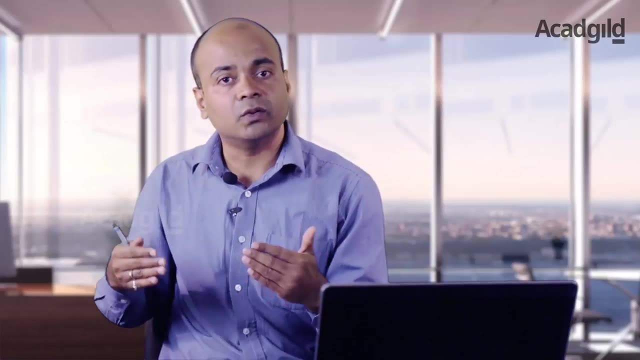 So that becomes inferential statistics. So the population in the state is going to be more than the population in the state. So the population in that case would be all the individuals of that, say, Gujarat, where people voted, And sample would be those people to whom you went and asked: hey, are you going?